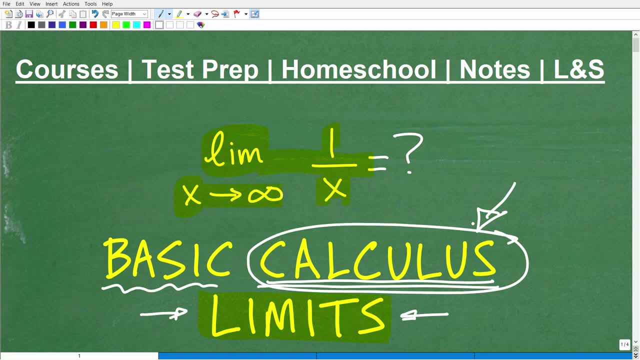 math for decades. It really is my true passion to help as many people as I possibly can learn mathematics. And I'm going to tell you right now: all of you can be successful in math. And I'm especially speaking to those of you that maybe have a fear of math or maybe you struggle in math. 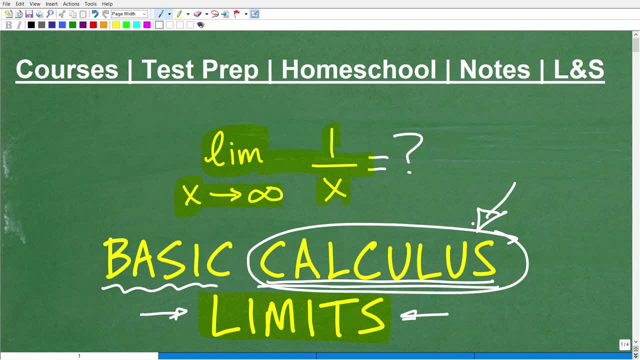 Listen, do not give up hope. You can absolutely be excellent in mathematics, But what you need is great math instruction. ie whoever you learn math from, or whatever you're learning math from- ie, if you're using some sort of video, you're going to be able to learn math, And I'm going to 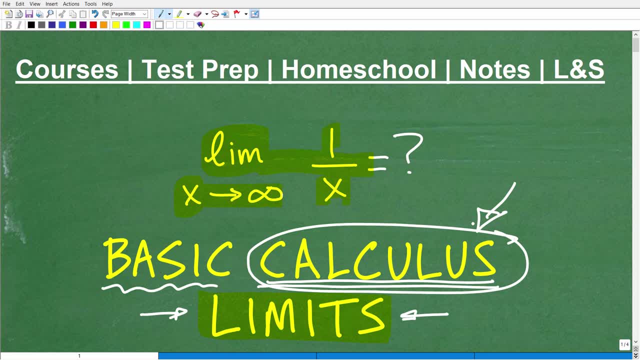 tell you right now, if you're using some sort of video program, textbook software, you have to understand what's going on. I mean, obviously, math is a very technical subject and it can be taught in a very technical way. Unfortunately, if you're being taught in a very technical, 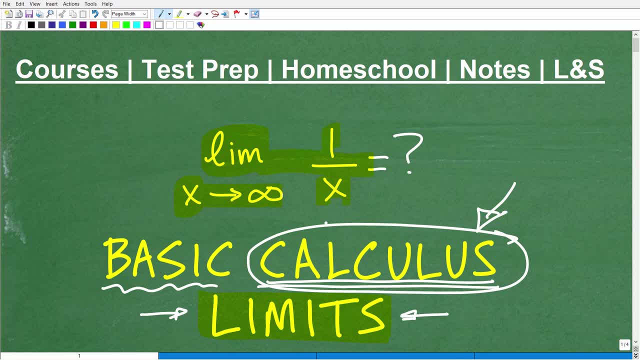 manner. it's confusing. OK, the way I like to teach math is to explain things in easy to understand language so everybody knows what's kind of going on without watering down what you need to actually know. So if you need help in your current math course or maybe some sort of 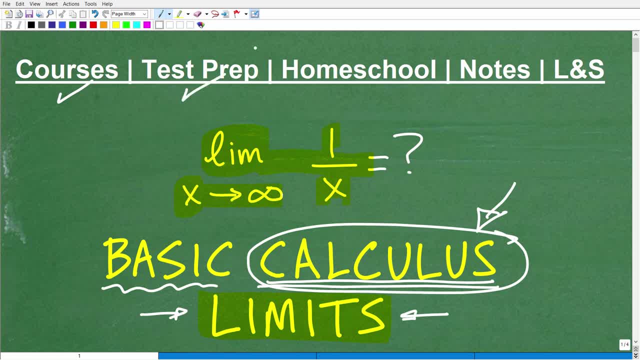 special test that you're getting ready for, something like the GED SAT, maybe a teacher certification exam. or if you're homeschooling mathematics, check out my math help program. I'm going to leave a link to it in the description of this video. I literally have over 100 plus. 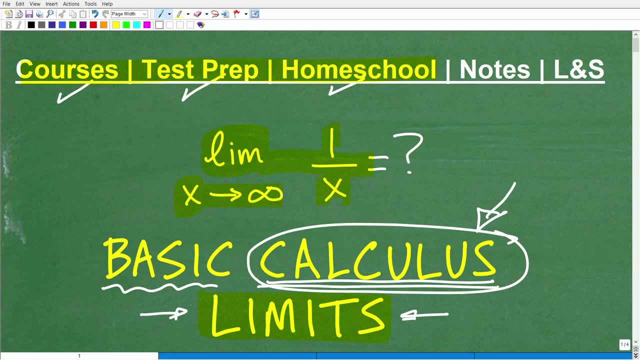 different math courses that span these categories and much, much more. Now let me just tell you right now: my highest level, most advanced course, is pre-calculus, So I do not teach a full calculus course If you have an interest in studying calculus ie. 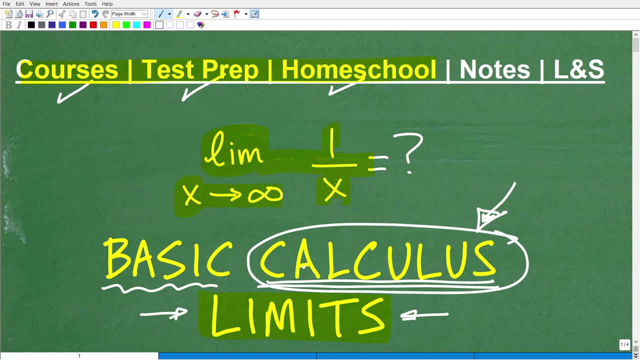 going to school for it taking a full course. I'm going to suggest that you look into going to a local college. you know something along those lines. Calculus, you know, is a very advanced math, but you, in order to take calculus, you have to get through pre-calculus to be ready. 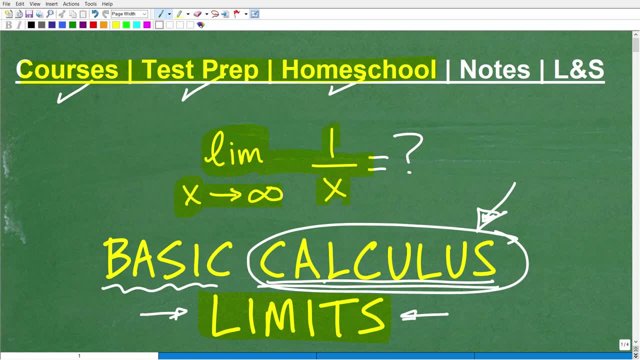 for calculus, So I do offer pre-calculus Again. you can just go to my website and check out all the information. Also, I want to leave links to my math notes in the description. You have to take great math notes to be successful in math, So improve your notes. 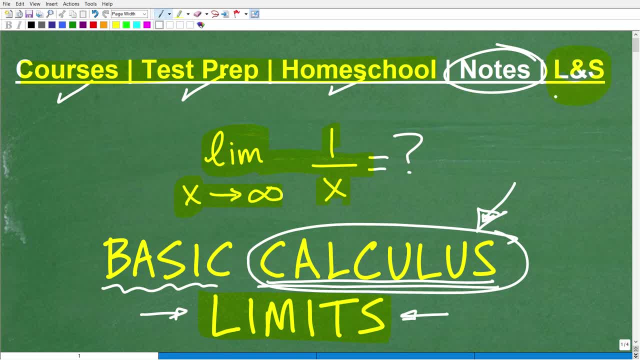 And things will get much, much better. if this video helps you out, Or if you like this video in some small way, don't forget to like and subscribe, as that definitely helps me out. OK, so let's get into this concept of limits Now. I mean, this is pretty crazy looking notation. 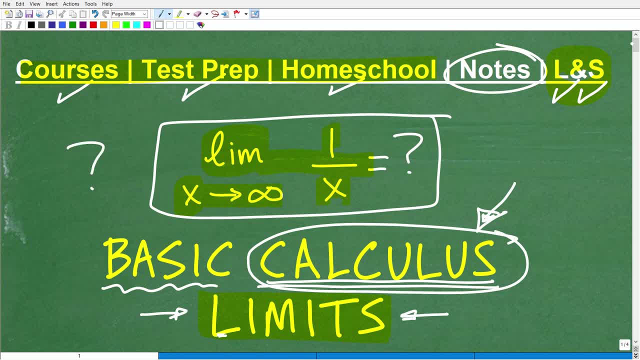 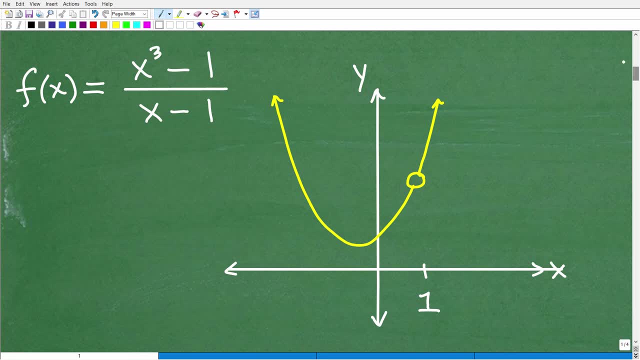 We're like: what does this mean? You know what is this all about? Well, let's kind of take a look at an example problem to try to introduce you to this concept of limits. All right, Now I'm going to explain something here and hopefully you have some. 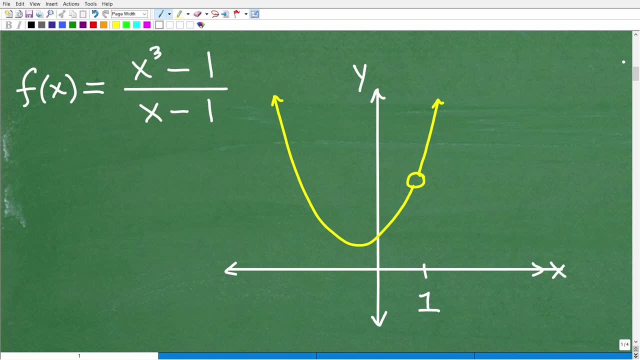 basics, Basic level, basic algebra knowledge. Right, I'm talking about, maybe like the algebra one knowledge. So what we're looking at here is what we call a function And again, if you've taken a course like first year- algebra, algebra one- you should be able to understand what 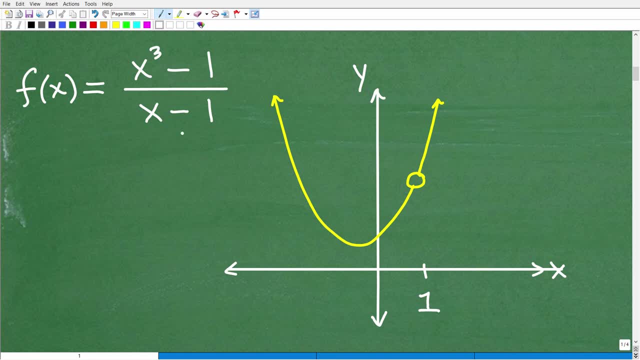 this thing is. Now, what I've done is graph this function. So this is more or less the graph of this function. Now, why this is the graph, that's a whole nother topic. But just kind of trust me, if we were to graph this, this would be the function And you can see, here we have. 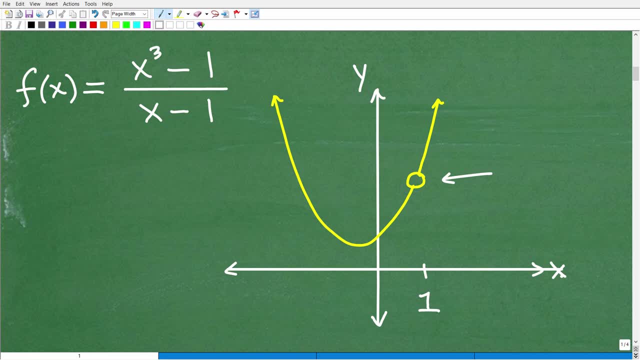 this whole right here. Okay, So here's the X axis, Here's the Y axis. Here at one there's a whole. Okay. Now, why is there no graph right there? Okay, Effectively, I can kind of just erase that. 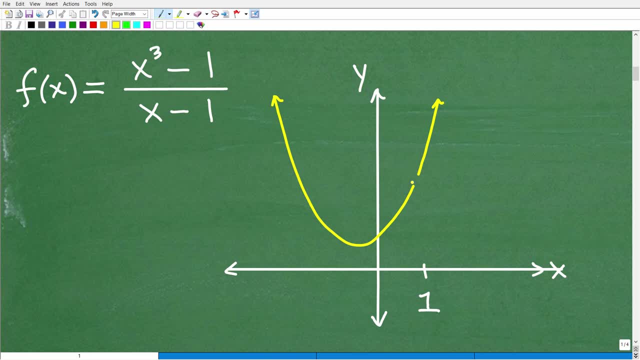 right there, That's like a missing part of the graph And like, hey, what happened to the graph here? It's missing. So we'll just put a little hole like that. Well, it's missing because at one. okay, right there, we cannot evaluate this function for one. Well, we could try. right, Let's see what. 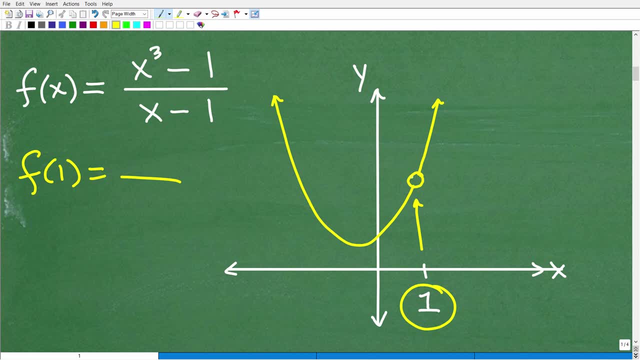 we try. So if we wanted to find F of one- ie this point right there- we would go one, We replace all these Xs with one and we got one cubed minus one over one minus one. And here we. 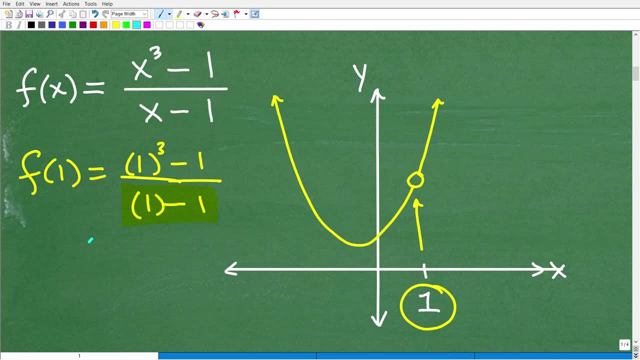 run into problems. This is a good way to blow up this function, And we don't want to do that, right? I mean, that's the last thing we need. So one minus one is what? Zero? Okay, So you can. 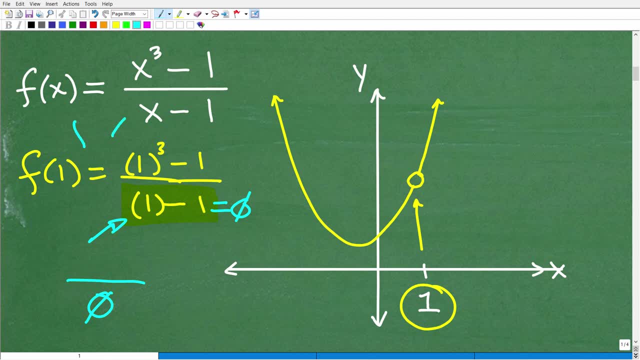 never have zero in the denominator. That will blow up your function and then you'll have other functions. So we have to restrict one from the domain. Okay, I'm kind of using some algebra terms here, Terms here, excuse me. So one cannot be part of the domain because if we plug in one again, 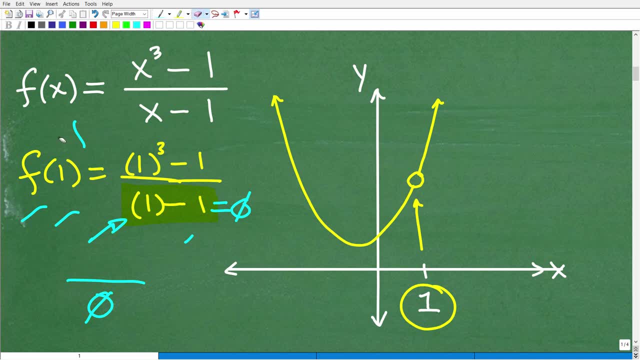 we're going to blow up the function and we don't want that to happen. All right. So again, because one cannot be part of the domain, ie the set of input values. when we graph this, we have to just show: hey, there's a hole here, There's no value because one is restricted from. 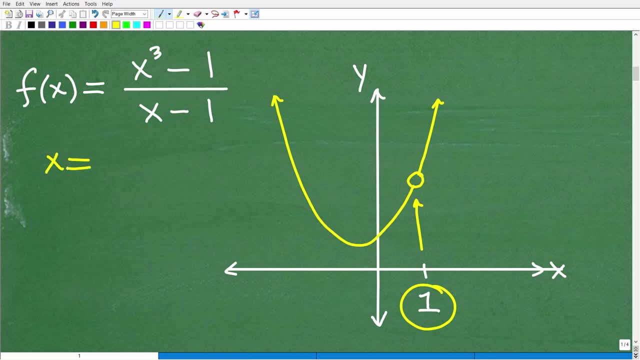 this function. Technically, I should put, x cannot be equal to one, for the reason why I just said: Okay, no problem. But here's the deal. You can see here, if we kind of look along this graph, if we kind of approach one: okay, we do have values here, right? So in other words, 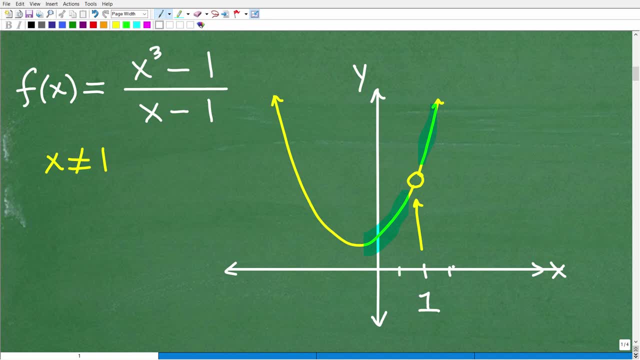 so right here, this is one half, this is one and one and a half and here's two. I mean there's values along this graph. What happens if we get like super close to one, In other words, as we approach one from both sides, what is the value? 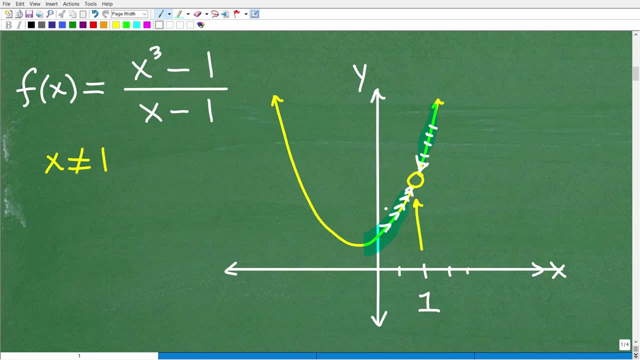 going to be right here. Now we're approaching from the left and we're approaching it to the right, So we're trying to get super, super close to this off-limit value. okay, So what is that actual value If we get infinitely close? imagine if we get like: really, really, really, really. 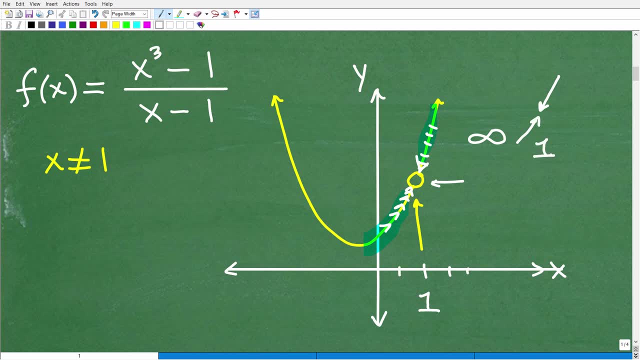 close from the left and from the right- Now we can't touch one- But what would be this value? okay, So this is kind of just a real kind of basic explanation of the concept of limits. What we're trying to do is to determine this value that, as if we approach, 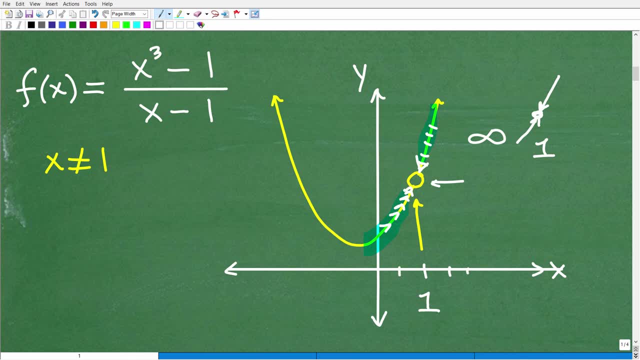 this one. okay, on this particular graph, as we get closer and closer to it from the left and right, what would be the if we got infinitely close to it? what would be the actual value? So we would try to find the limit. okay, So that's what this is called. 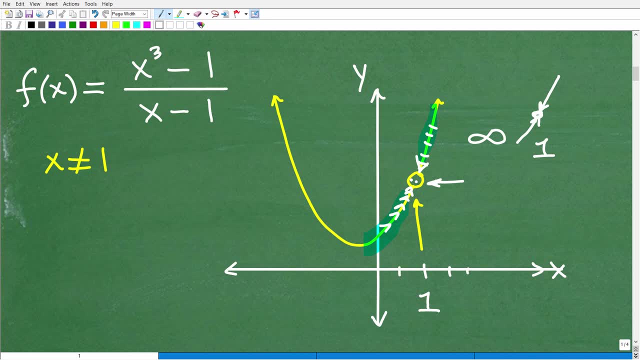 We're trying to get the actual value right there If we get infinitely close to it, but we don't touch it. All right, so hopefully that basic explanation makes some sense. That is the whole idea of limits. Now, when you study calculus formally, there is a lot to this. There's this: 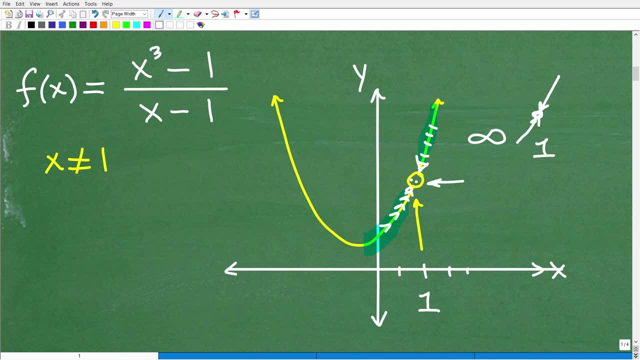 stuff called epsilon and delta and there's a lot of rules to limits. You know, if you take calculus, if you're intended to be a full, you know, enroll in a full calculus course, you'll learn about this. So this video again is intended just to give anyone out there, even those of you. 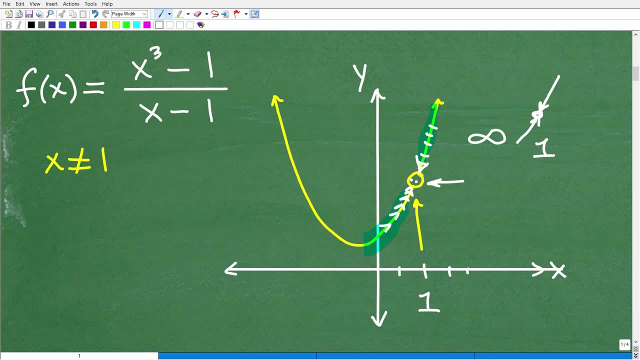 that have no intention of taking calculus, just a basic flavor, a basic sense of what limits are about. So let's go ahead and take this to the next level, So let's try to determine what that value would be okay as we approach one, from both the left and right. ie, we want to find the limit. 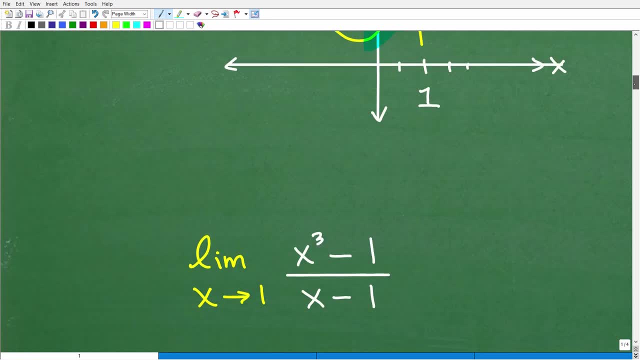 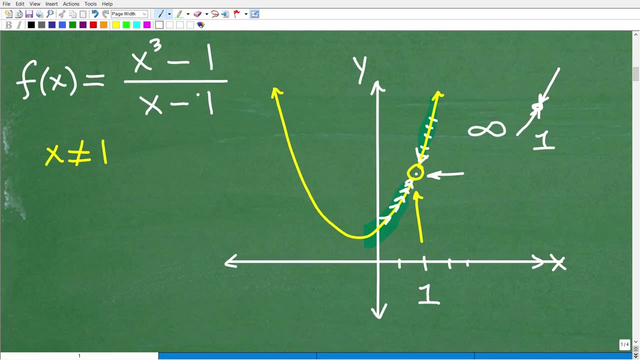 of this function as it approaches one. okay, So we would use this fancy notation. So here you can see. this is our uh function. uh, f of x is equal to x cubed minus one over x minus one. So we can write this: 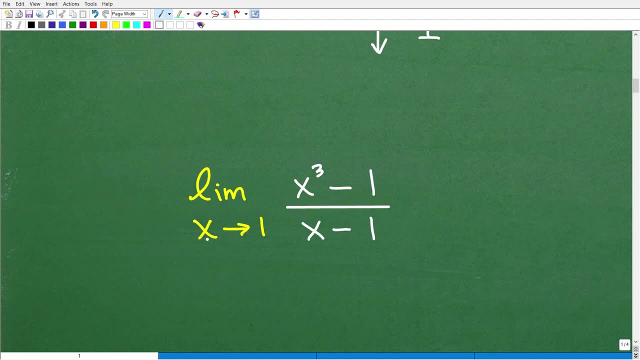 fancy notation right here. So we want to find the limit as x approaches one. okay, Now you could approach a function from the left and right. Again, I'm just going to leave. uh, I'm not going to get overly technical for this quick introduction to limits, but basically we can write this right. 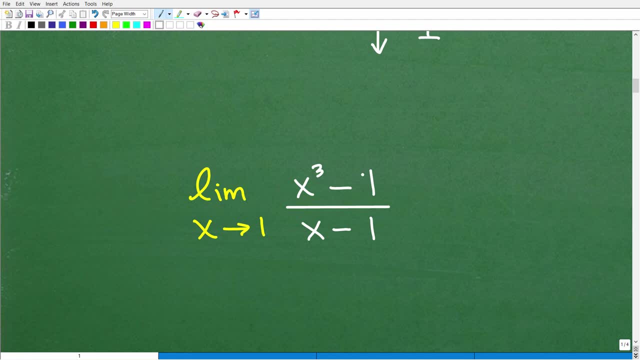 here. So what is the value of this function as x approaches one? Of course x can never be one, but what it would be? the, uh, you know what? what number, what value is it approaching from both the left and right hand side of the graph? Well, if we want to figure that out, we would do. 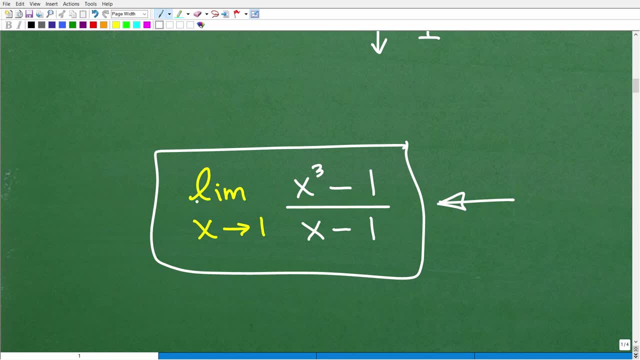 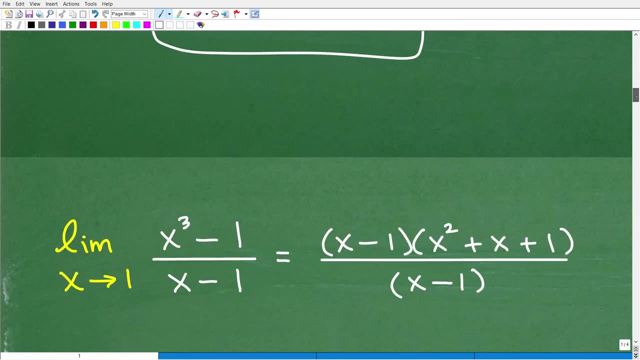 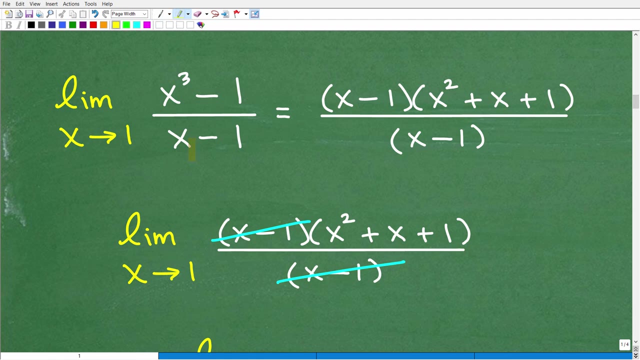 this, We would find out. we would want to ask the question. all right, what's the limit as x approaches one to this function? So now let's go ahead and talk about how we actually answer this question. Okay, so what we have to do is use our algebra knowledge. okay, So again, you're taking 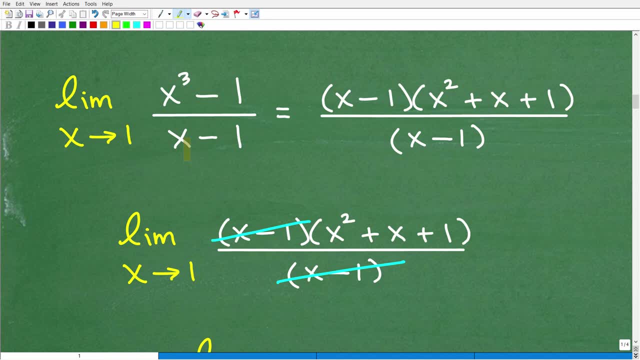 some strong algebra skills, certainly, um, you know, a requirement. but here this x cubed minus one, this is actually something called the difference of two cubes, and we can use our awesome factoring skills to factor x cubed minus one this way. So the x cubed minus one is equal. 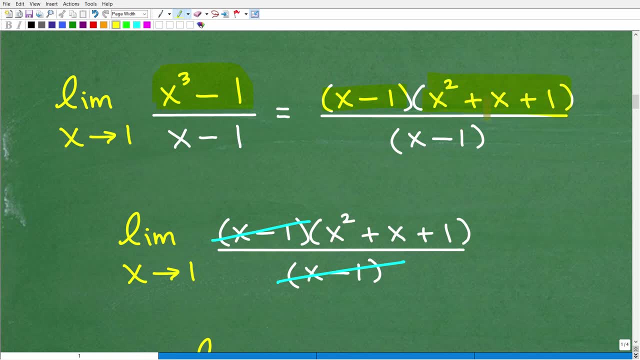 to x minus one, times this trinomial x squared plus x plus one, and then we have that over x minus one. Now, the lovely thing about factoring this function this way is that these x minus ones, uh, these factors, uh, cross cancel okay. So we want to. 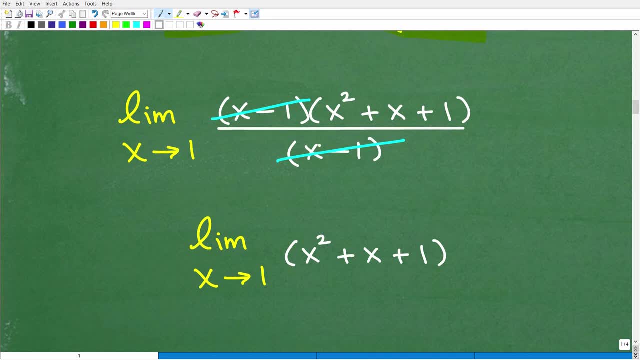 kind of use our algebra skills and get rid of um fractions if we can. There's all different sorts of techniques to evaluating the limits of uh, respective functions or various functions. So here is an opportunity where you can factor, definitely factor- and simplify uh that function. 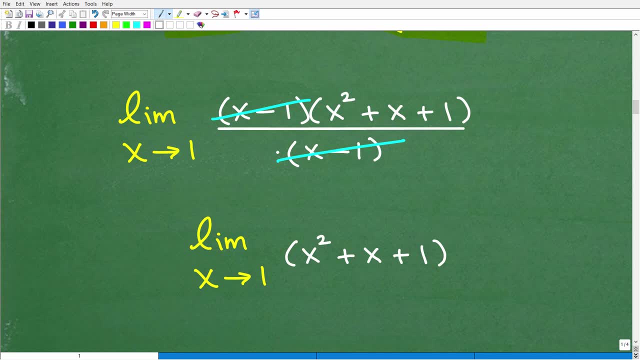 that you're looking at. All right, so we're going to cross cancel these factors so effectively. uh, our problem is now down to this. You can see how we cross cancel this. Now we're going to find the limit as x approaches one of this trinomial here. So how do we do that? 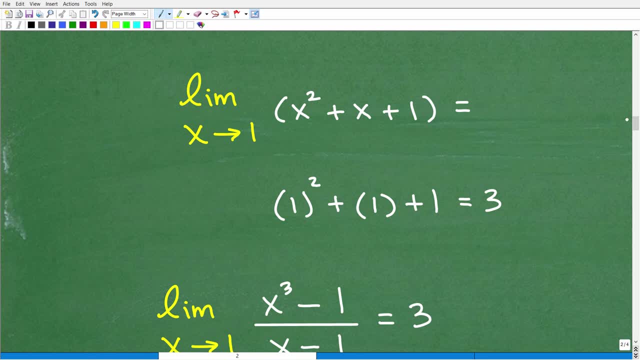 Well, there is a basic um kind of theorem, a uh law property, that you learn in calculus, but I'm basically going to simplify it. When we're finding the limit of a constant value, in a situation like this, it's literally as easy as just plugging in this number. okay, So this number one. 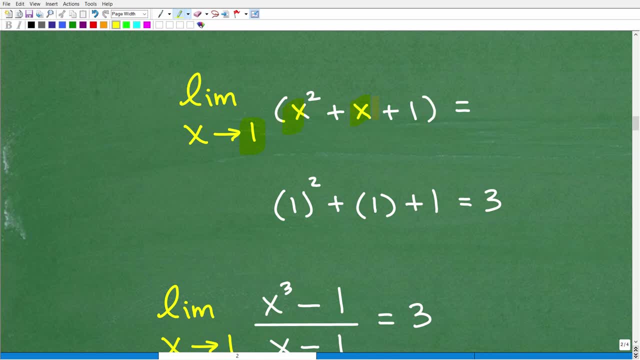 we're just going to plug in this number. okay, So this number one. we're just going to plug in this to this: um, uh, function. Now here we have no denominator, no restrictions on this, like x minus one, So we can plug in one right here, not a problem. So that's going to be what one square. 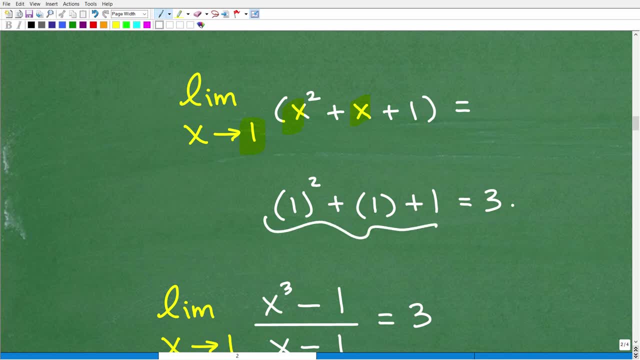 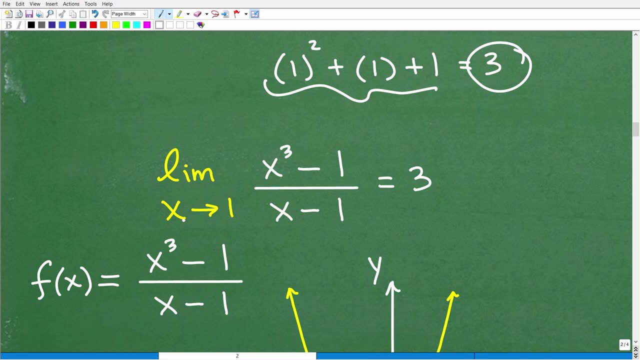 plus one, uh, plus one. So when I do all this, you get three, and that is the answer. Okay, So effectively, the limit as x approaches one of our original function here is three. Now, what does that mean? Well, let's go back and take a look at our graph right here. 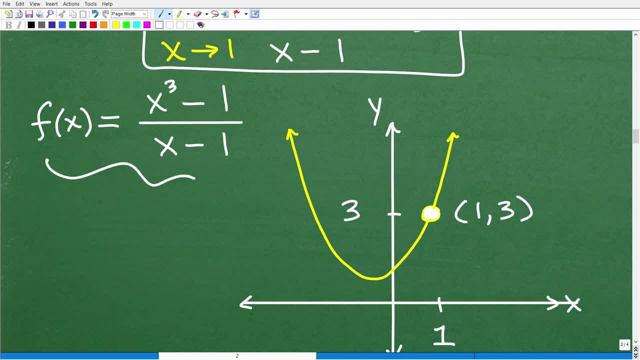 So recall that our graph had this hole in it at one, but effectively, as we get closer and closer to uh one on this function, from both the left and right, we're going. we're getting super close to three. Okay, That's basically what it means. So this coordinate right, there would be one. 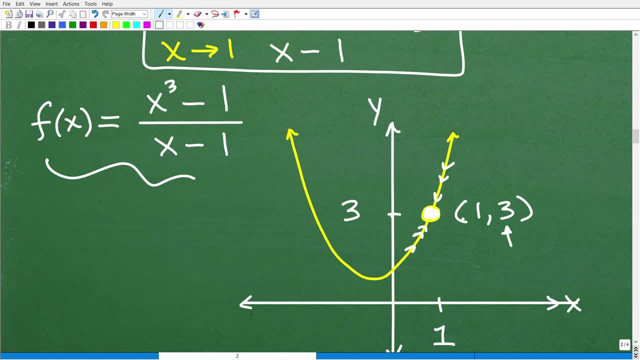 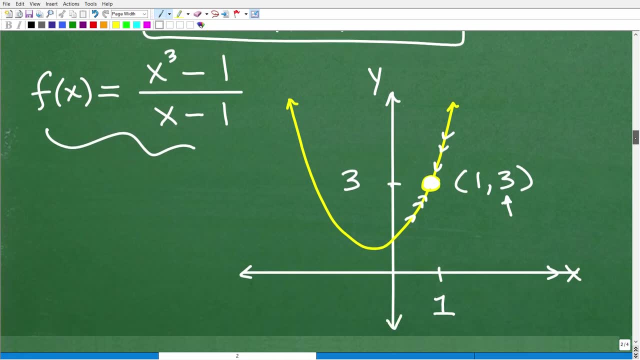 three. Now, of course, we can't ever touch it with that one, but that's effectively what that means, Okay, So hopefully that you know makes sense to you. This is a basic limit problem. Let's talk, uh, about finding the limit when something is approaching affinity. 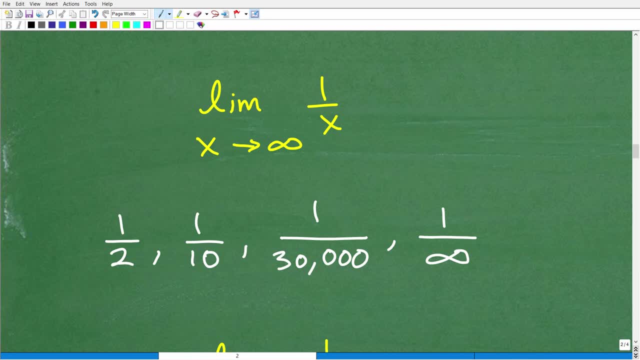 Okay, So we can uh. the last problem we talked about was the limit when a number x was approaching a constant value, like uh, three or one. but what happens when x is approaching affinity? Well, infinity, excuse me, not affinity. Affinity means, uh, a pretty uh. 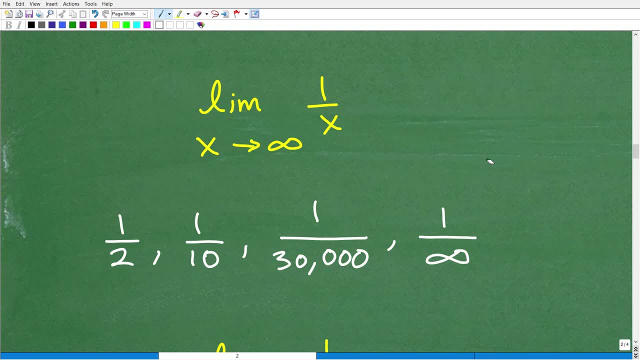 let me um, because I said the word affinity is like you'll like something, right, That's pretty much it. Or you have an affinity for something, So hopefully you have an affinity for an affinity infinity. Uh, you know, I should just really stick to the math, because my jokes are. 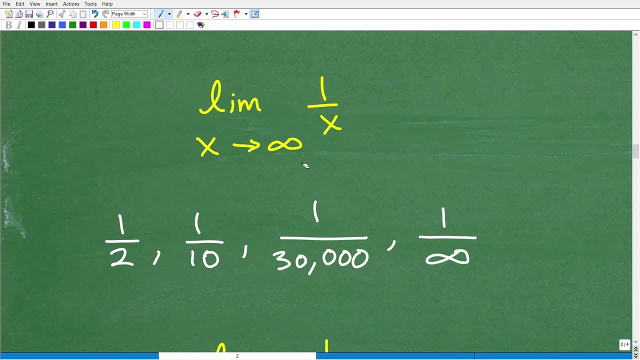 not that good, but anyways, you know, we're trying to make this an easy going video, All right. So, anyways, uh, we have the limit as x goes to infinity, one over x. So what does that mean? Well, let's, uh, you know, let's just kind of think about this for a second. And infinity is. 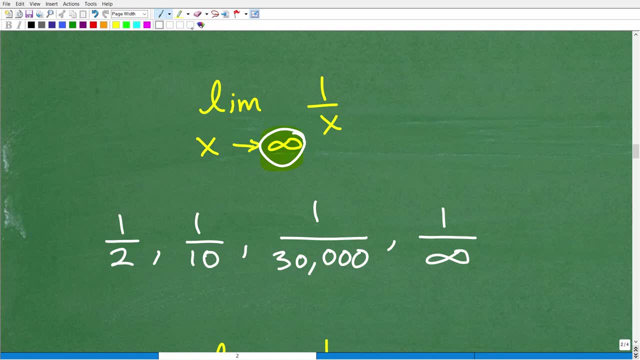 very large number. right, This is a big number. So one thing you've got to do is like: all right, we have one over the biggest number in the universe. right, One over the biggest number in the universe. That's what x is approaching to. So what is kind of going on here? Well, 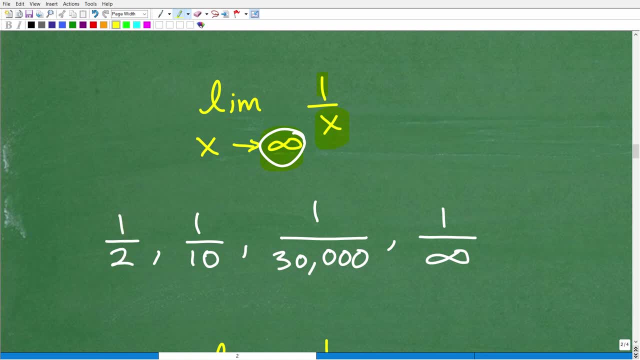 let's just start looking at some patterns of fractions as the denominator gets bigger and bigger and bigger, And of course this thing is going to get infinitely big. So here we have one half, All right. So let's just start increasing that denominator. 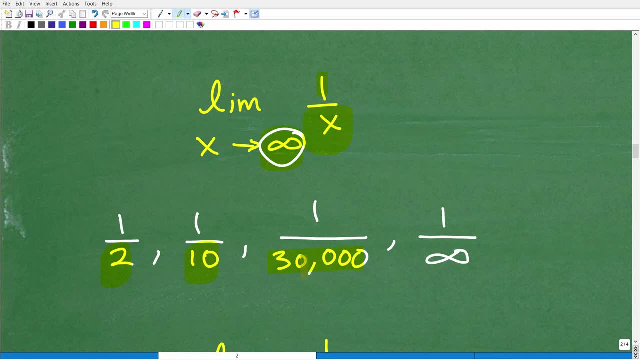 One 10th, And then we have one over 30,000.. What's going on with these values? right, Like, if you're comparing the values, well, hopefully you recognize that this fraction here is much, much smaller in terms of value as this number. So as we increase the denominator, the overall 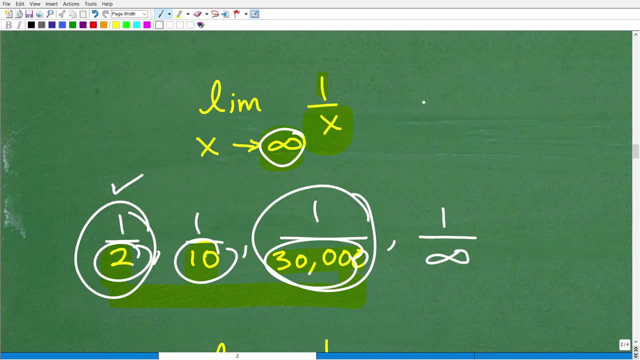 value of the fraction is getting smaller and smaller and smaller, right? So here, for example, here is one, here is a zero. Okay, As we increase the fractions or the denominators here, right, We're going closer and closer to. 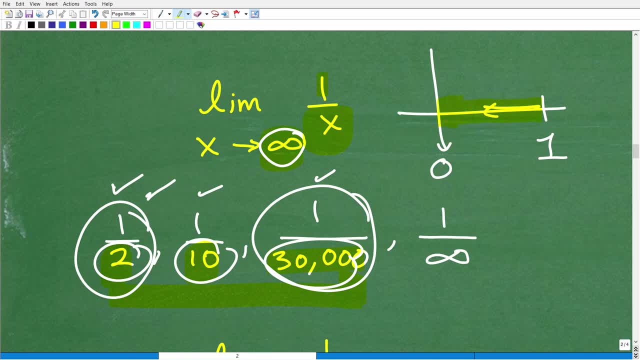 what Well we're getting close. We're basically decreasing the whole value of this thing. Okay, We started off here with one half and then we're kind of you know, really getting down over here. But now I want you to kind of guess, right, What do you think is going to happen when? 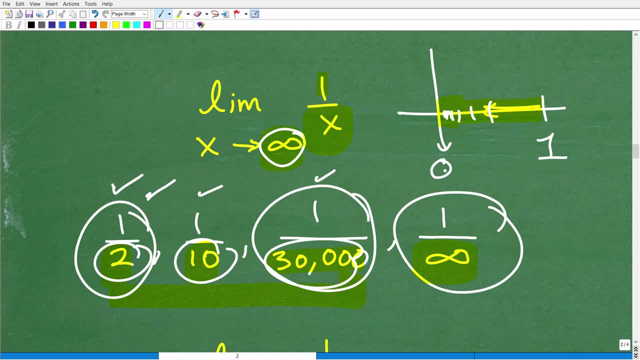 we take that denominator, We make it infinitely large. Where are we approaching? Okay, What value are we approaching? And I'm kind of giving you a hint, right there, Right. So, hint, hint, hint. If you said zero, you would be absolutely correct. So we have this. 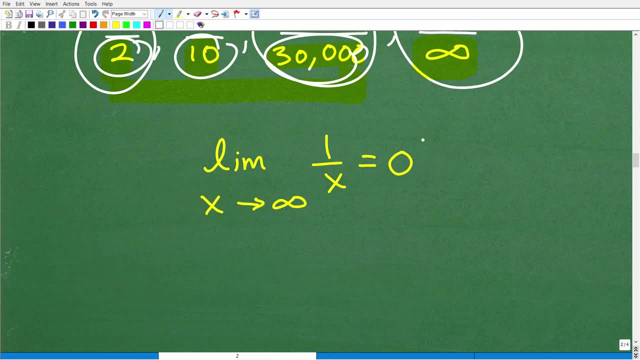 basic rule here: The limit as X approaches infinity, one over X is zero. Okay, So this is pretty much a very basic kind of rule or property when you're studying limits where a value is approaching infinity or infinity, excuse me, So in calculus, when you're talking about limits, 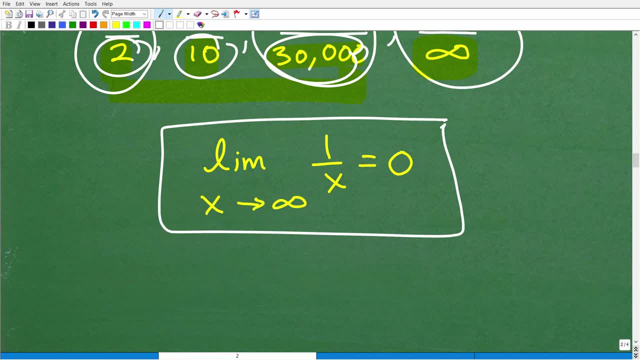 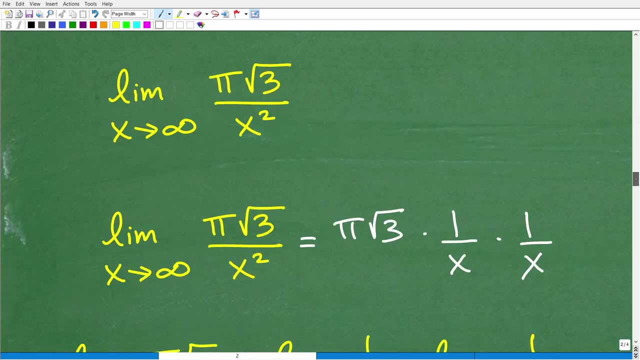 you're talking about when values are, uh, approaching a particular constants, And then you do a lot with infinity as well. Let's take a look at a quick problem, and then we'll wrap this up. So here let's figure out this function. 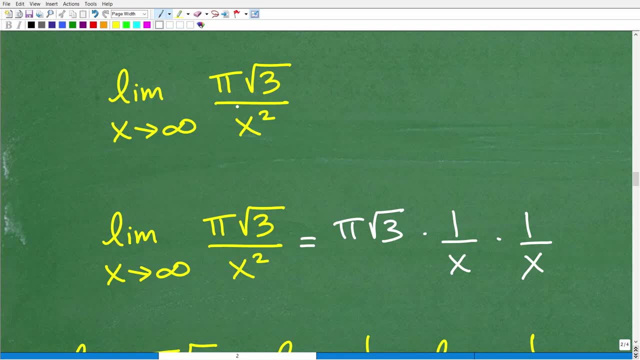 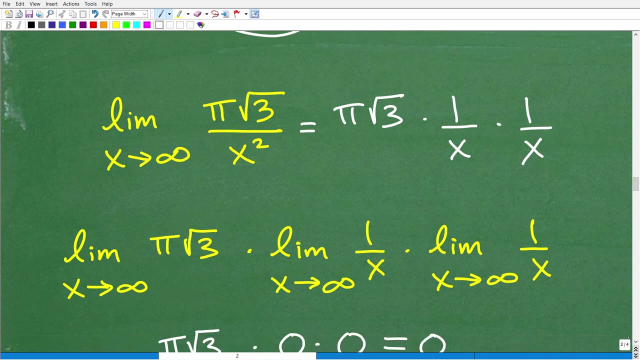 the limit as X goes to infinity, we have pi times the square root of three over X squared. So to figure this out we have to use our awesome um algebra skills. Okay, So you can see. algebra is coming up over and over again in calculus. All right, You have to be super strong in a high. 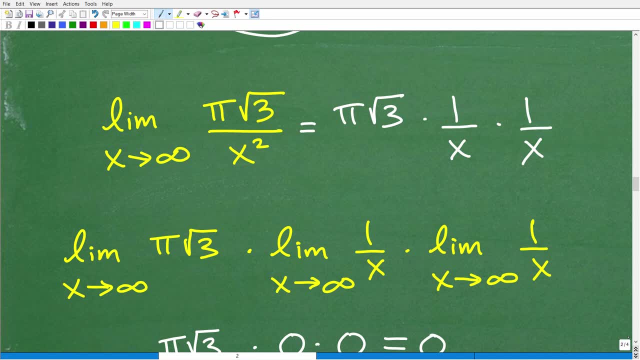 level mathematics to be successful in algebra. Now there are some high school students that take AP calculus. I'm sorry, Uh, yes, Let me just make sure I said this right: You have to have super strong algebra skills And that's why you know being, um, you know, successful in a course like 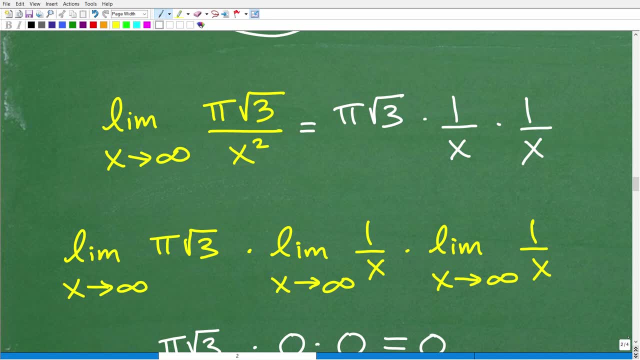 pre-calculus is going to set you up for success in calculus. So if you struggle with- you know high school level algebra, algebra one, algebra two, you know college algebra, pre-calculus- you're going to have a tough time in calculus because you're going to need all those. 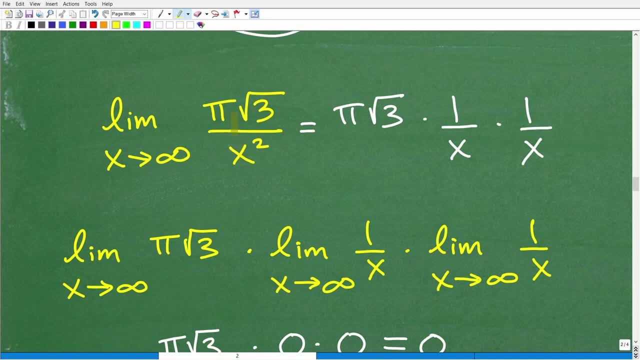 strong algebra skills. But anyways, what we can do here is factor this. So we need to look for creative ways to factor this expression. So we can factor this this way: pi times the square root of three times one over X times one over X, because one over X times one over X, this right. 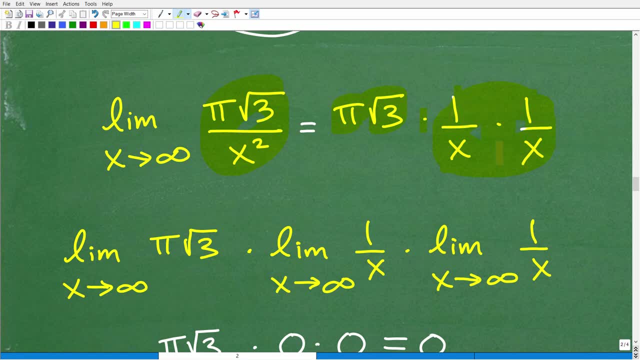 here. if I multiply this together, this is one over X squared, one over X squared times. This gets us back to this. but I want to kind of factor all this out And then what we're going to do is take the limit of each of those factors. That's another rule that we can do. So we can. 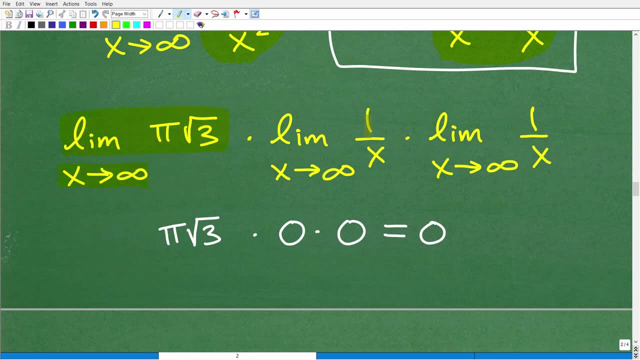 find the limit of the first factor as X goes to infinity. And then we have the limit of the second factor, which is one over X, as X goes to infinity, And then that's going to be multiplied by the limit of one over X, as X goes to infinity. Now, when we're, um uh, looking to evaluate a limit, 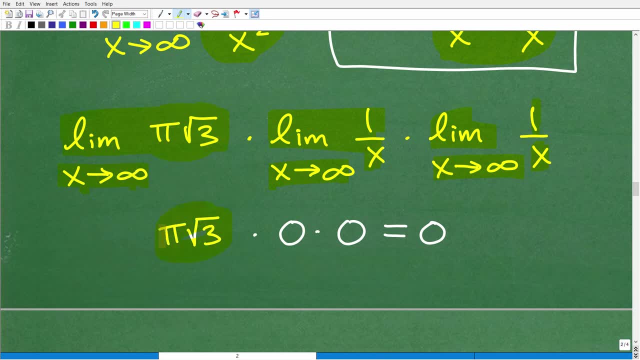 as X goes to infinity of a constant. it's just simply going to be that number Here. we just figured out what the limit, as X goes to infinity, one over X, right? We just went through that and we that's going to be zero, right? Cause our denominator is going to be: 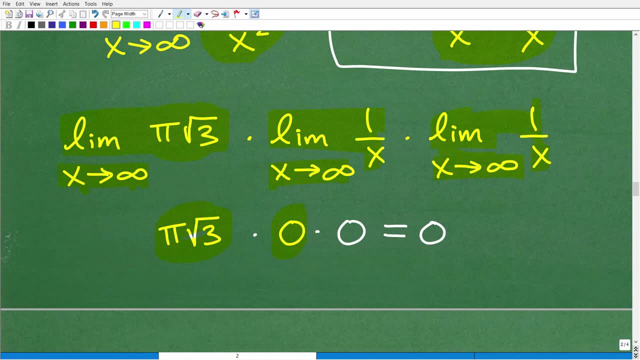 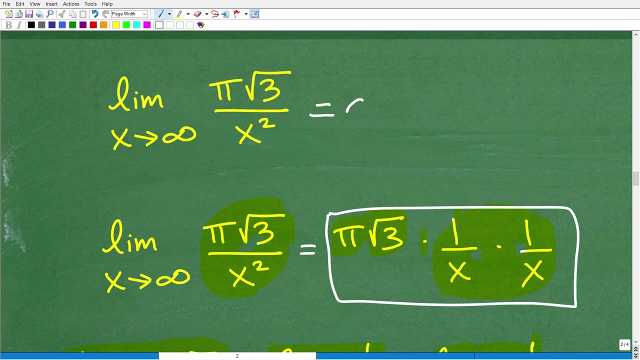 infinitely large. So when we evaluate this limit, that's zero. And then this one right here is also going to be zero. So zero times zero times, pi times, the square root of three is what? that's just going to be zero. So our final answer here would be zero. Okay, So calculus is a awesome. 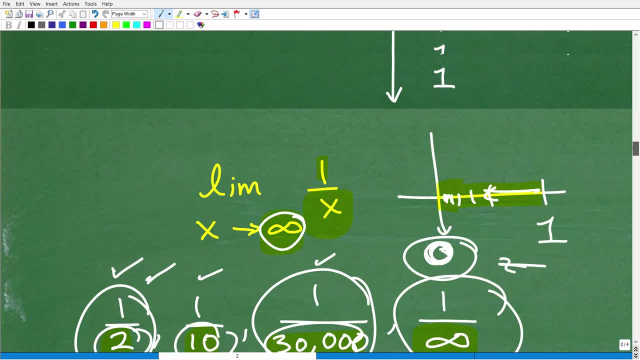 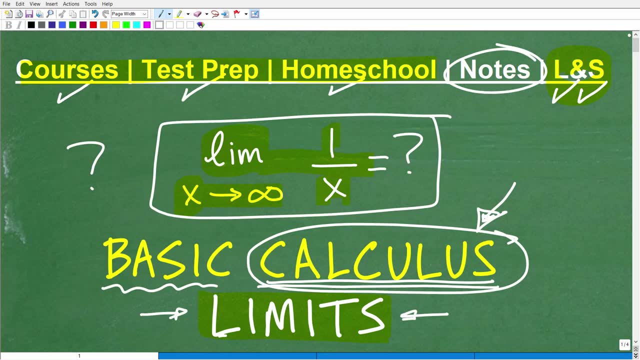 course. I mean there is a ton to learn. but you know, what I try to do with these videos is try to, you know, get those of you out there that are interested in calculus, excited about the concepts in calculus, And 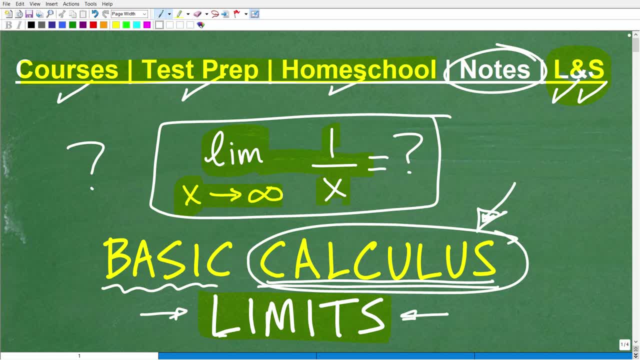 you know, I try to really really, uh, give you these really, um, kind of basic introductions to some of the meanings of calculus. Now, if you happen to be a calculus professor or whatnot, you're like: well, you're missing this, You're missing that. You should have said this Well. 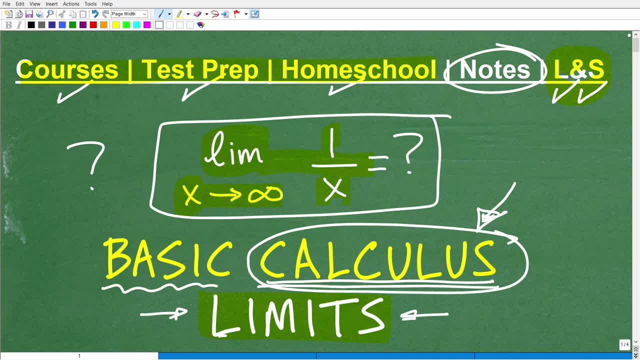 let's not get that. but this is not designed to be a formal calculus lesson. You know, uh, you know- those of you that are going to actually be taking the course- we'll get all that kind of good stuff. But, uh, even if you don't take calculus,